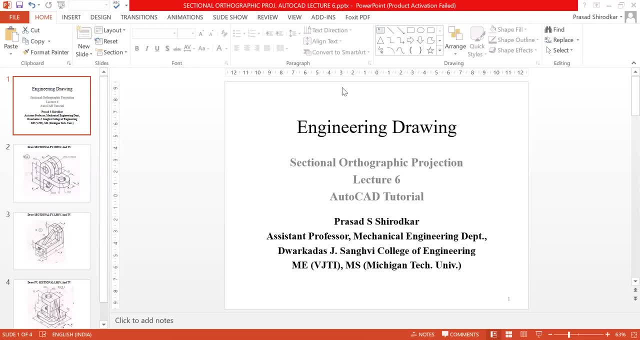 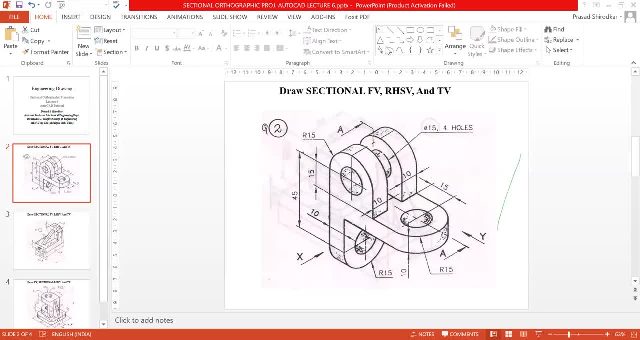 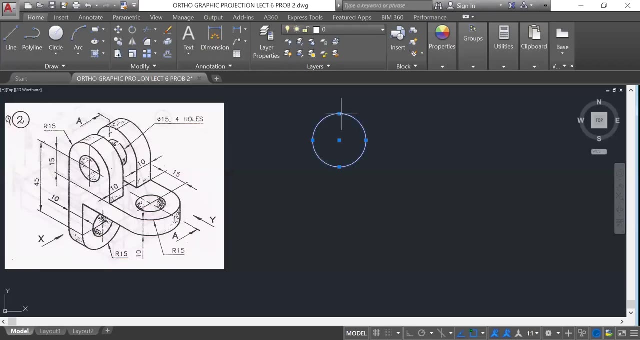 Thank you. Thank you. So we are going to solve sectional front view For sectional front view, right hand side view and top. So we are going to start with the solution. So we are going to start with the sectional front view. So to start with the sectional front view. 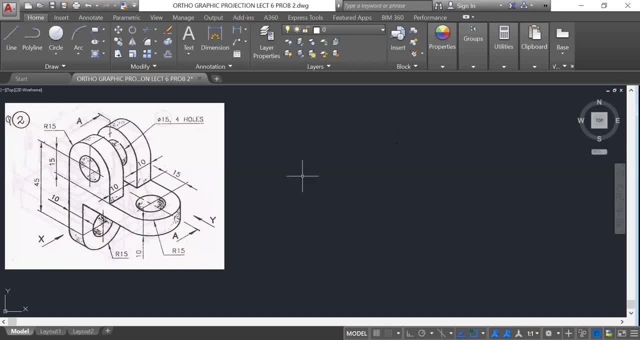 first I am going to, First I am going to start with the circle. The radius of the semicircle is 15.. So pick the circle command, Click somewhere in the screen, Type in 15. 15. 15. 15.. 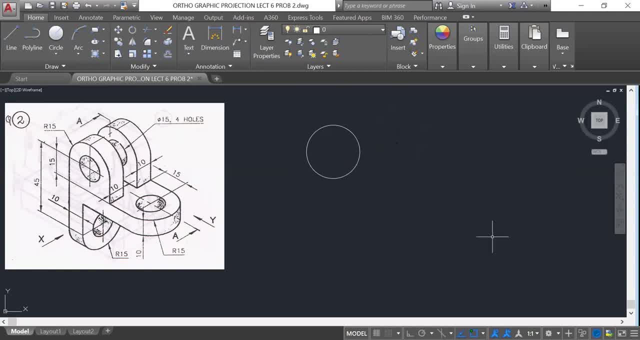 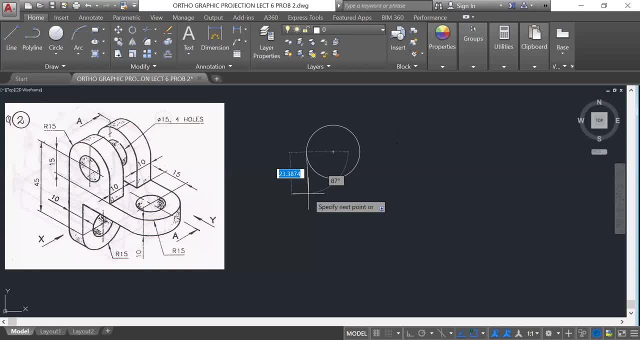 Select the butden Go down Type in 15 and then in horizontal Type in four together kauarmaelez to produce A union퀸 Again. sign over to the line from the second for wieder: go, go, go, go go. 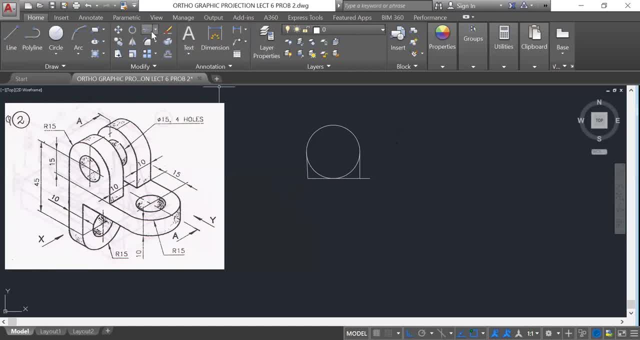 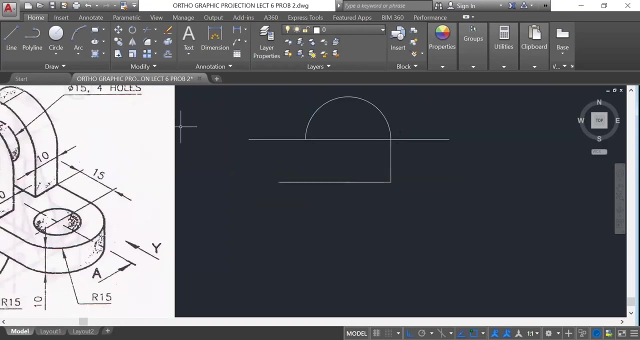 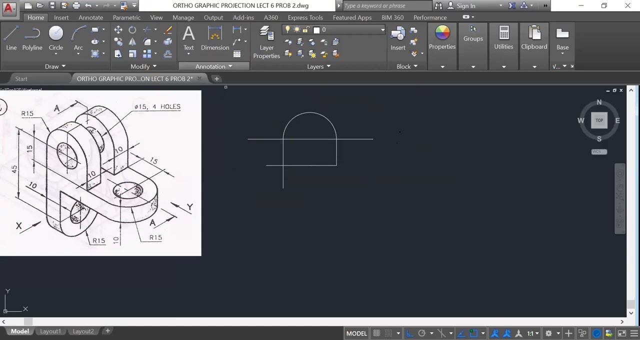 Now we will. the second will construct this plate. So this is the first part. this is the second. error wasn't used to fix that. Go to the trim command and trim the excess. Okay, So that completes the first part. Now we'll do this second plate, which is horizontal. 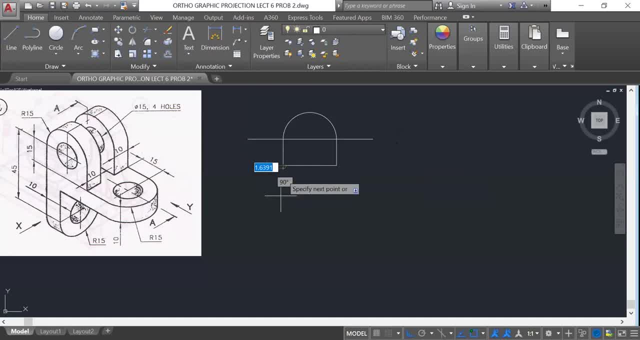 So for that, click on the corner, move down equal by the thickness. thickness is given as 10, type in 10.. Okay, then width is radius is 15.. So it will be 30.. So type in first 30, enter, then again 15. more, type in 15, enter and again the radius. 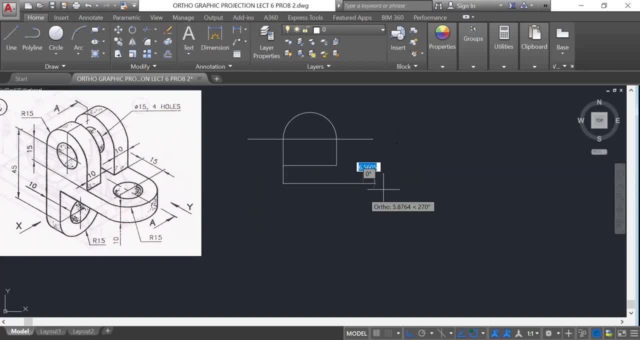 of this, of the second is also 15.. So again, type in 15 and move up, type in 10, enter and close it. So total width is 15 plus 15, that is 30 plus 15.. So it should be 60.. So let's just check. 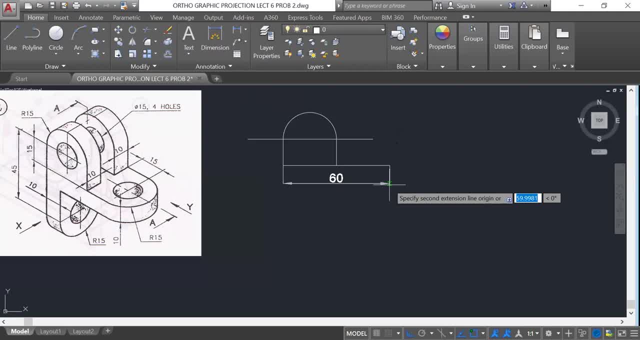 the dimension, It is 60, wrong Always. you have to check in this one Then. then we'll construct this second vertical plate. All right, So vertical plate, This third vertical plate is: we have to check. All right, So vertical plate is the three. 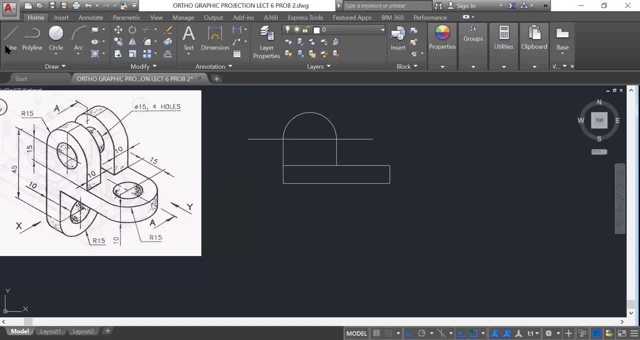 vertical plates plate. it is of. again, from here to here it is. from center to center, it is 45 and from the top edge it is. so I'm just going to do that from the center line, just drop a line and type in 40, 45 for the center line, and after that it goes. 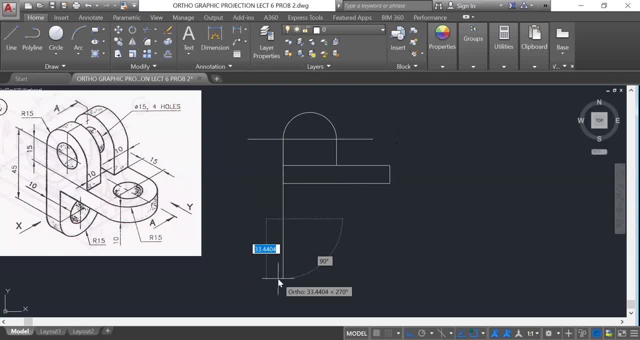 15 down more right and again the width is 10, enter and go up and close it. I click and enter. all right. now, when you take the section through the section plane AA, the material of this horizontal plate and this vertical plate is on the same plate. okay, so that entire two plates are cut, but this two vertical. 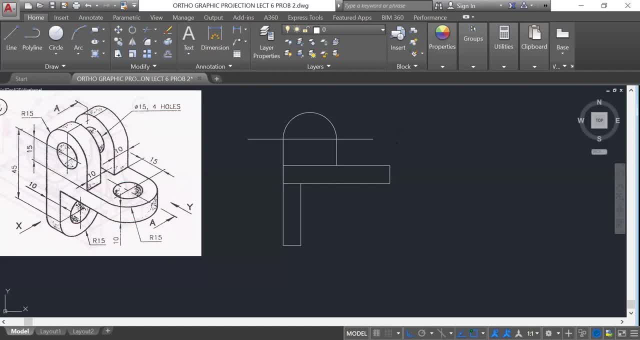 plates, the one. there is a gap in between these two, so these two plates are not getting cut all right now. once you draw this outline, you also have to mark the two slots. it is one and the horizontal or the center. so to mark the slots, the offset type in 15. 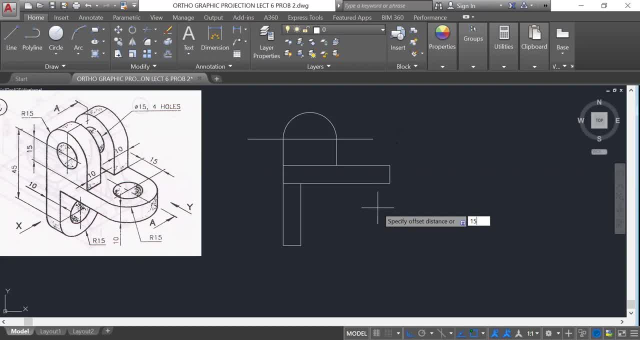 52 into two more. want to equalize these two holes. 13. bring this third one on to the top7 cross cross R 15. enter and take the object 1. take this object also, right click, enter. and the diameter of this lot: five fifteen four holes. all right, so again to offset. so diameter is 15, so radius will be 7.5. so type in 7.5, let enter, select one stars, so that will be intercepted. now I justly worth innovative signal because I crying I'm supposed to intercept just like that. the diameter is 15, so radius will be inside of 9 pm. 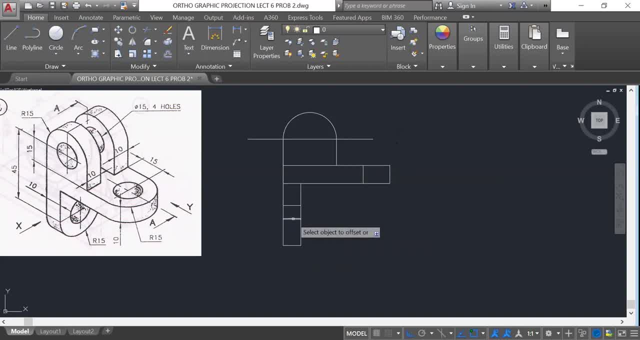 select one line, another line down, pick one line left, one line and right. do right click and all right, extend this little bit. all right, I'll go to the trim command now. since this entire material is on same plane, this line will not be there. let this thing come on. so that is your sectional front view now change. 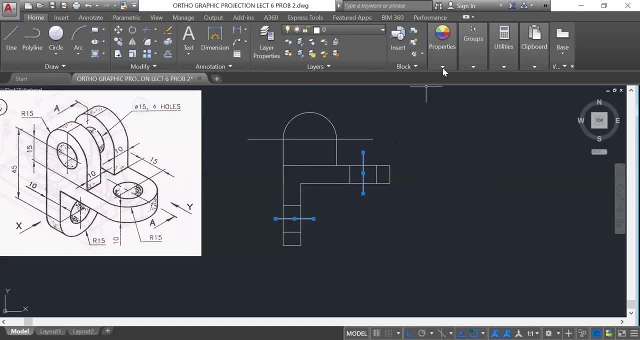 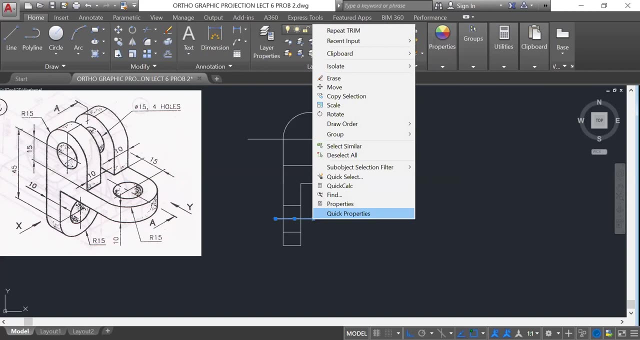 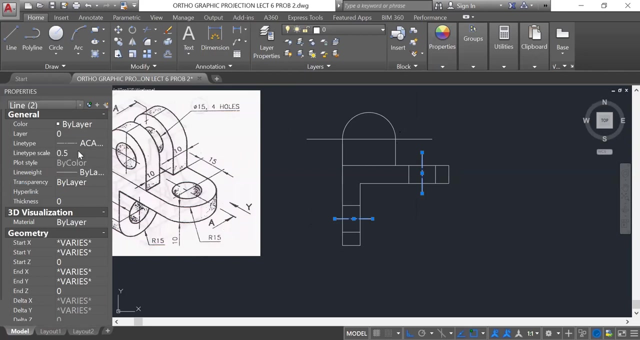 this to center lines: scale to 0.5 so that it is. reduce the scale to 0.5 so that it is properly this. all right, also draw a center line over here, so horizontal and one vertical center line match properties. take the center line and 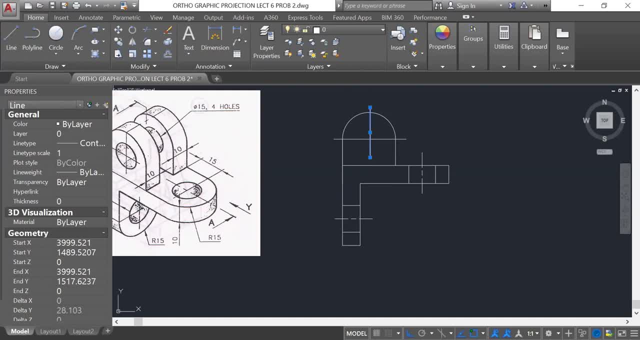 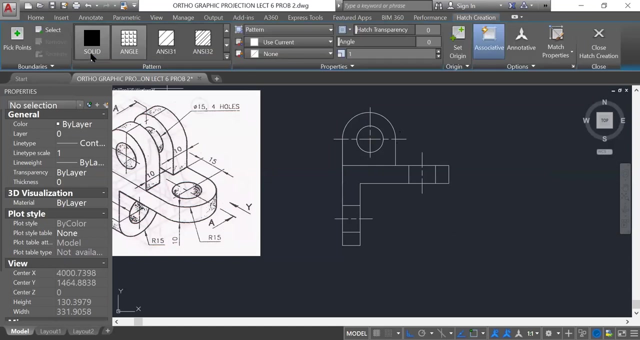 match properties. pick the center line, paste it, all right, and here also there is a circular slot. so at the center line, center, draw a circle of 7.5 mm radius, all right. after this is done, do the hatching, select the hatching hatch command, select ANSI 31 and pick the areas next one and two and the 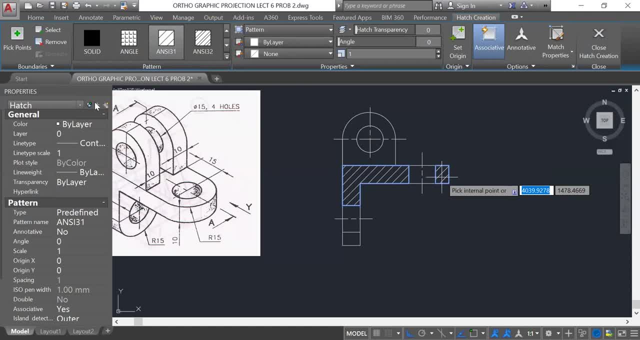 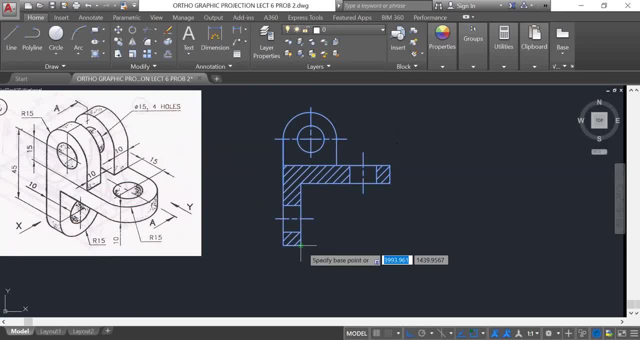 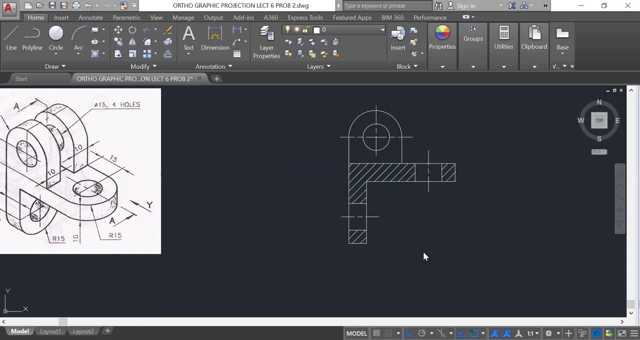 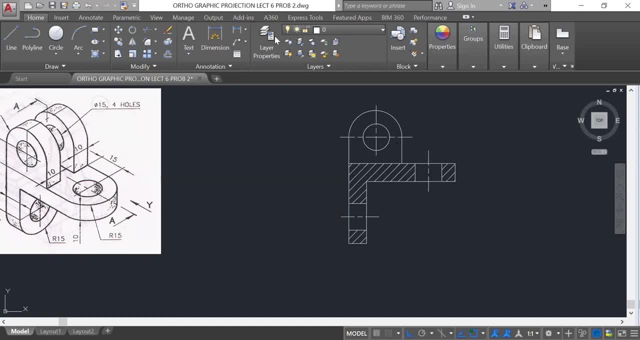 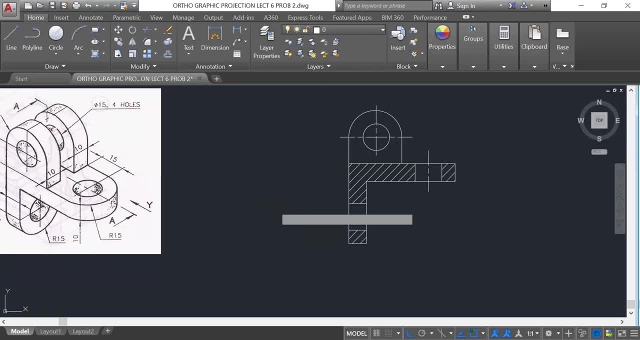 as we always do, keep a space. offset 20 mm over this stretch this up and horizontal projector and total width will be 10, will be equal to R 15, so total will be equal to 30. so offset this by that completes the block and it's going to trim whatever is not necessary. 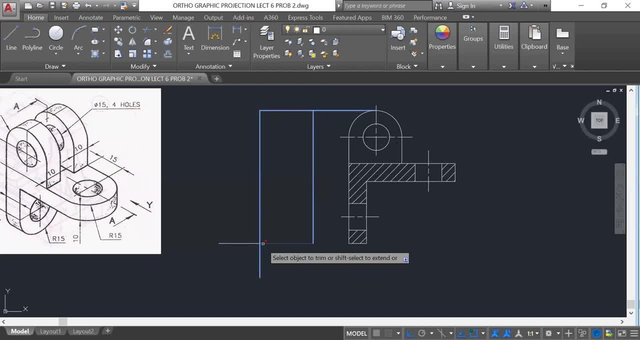 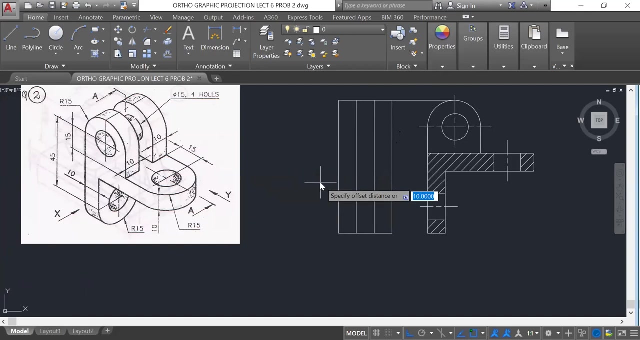 one, two, three and four. okay, okay, all right. so one by one we are going to start. so let's make these two vertical plates. okay, so go to offset, type in 10, enter one, two, enter and again go offset. then total height will be. height of this plate will be 15-15. so that is 30. so type in 30. 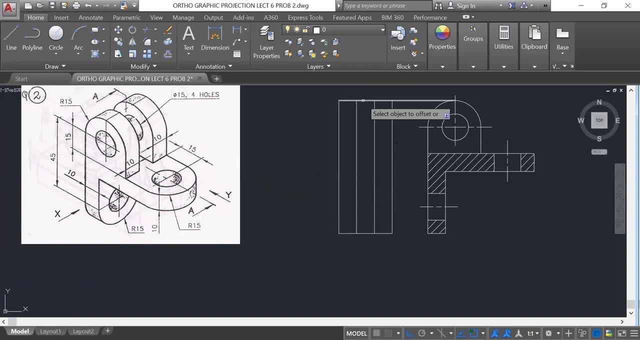 enter the topmost line and right click. enter and go to go to trim. click this line, right click and trim this line right. trim this line also, all right, and then also make this circular slots. trim this line also, all right, and then also make this circular slots. 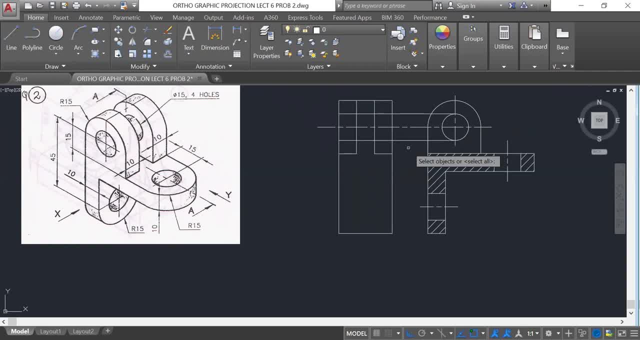 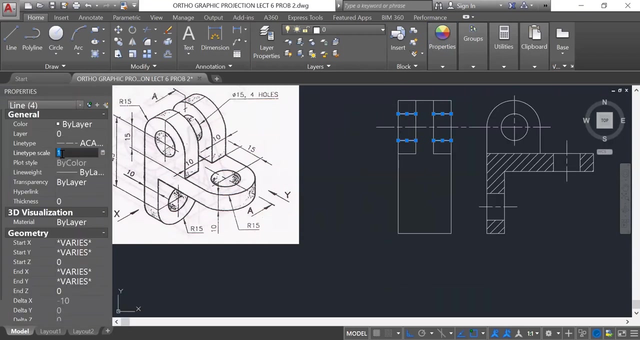 trim command, trim command, trim command, okay, okay, and this will be hidden. take this four lines and change them to, and change them to continuous, to theta now for this. change it to 0.5 and change it slightly to 0.2, and then do the match properties. 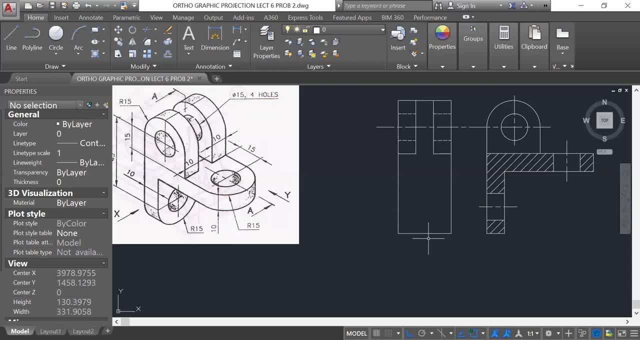 alright, so that completes the first two plates. now we will construct the remaining parts. for this second horizontal plate, we will draw a projector and one more at the top and then just trim this and there is a vertical slot in this horizontal plate. so I am going to construct a centerline. 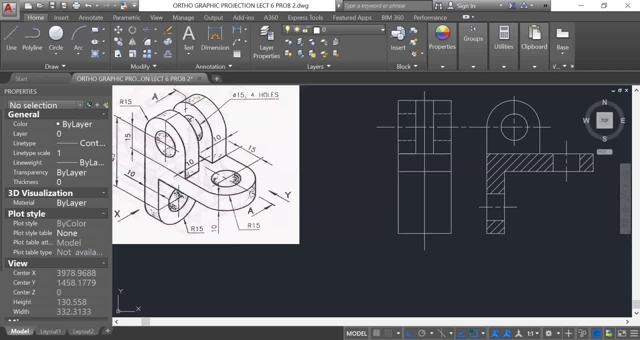 centerline should be slightly larger than the outline and then offset it on either side. so radius is radius of this slot is 7.5, diameter is 15. so 7.5 enter, offset 7.5 enter. take the centerline and click on both the sides. 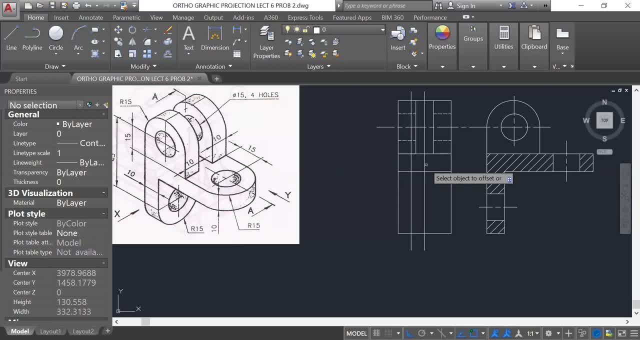 1 and 2 enter and then just trim this line 1 and 2 and right-click trim, trim, trim, trim, right-click trim, end. now we will just change some properties. these centerlines, this vertical one, is centerline- right-click enter and then for the hidden lines, 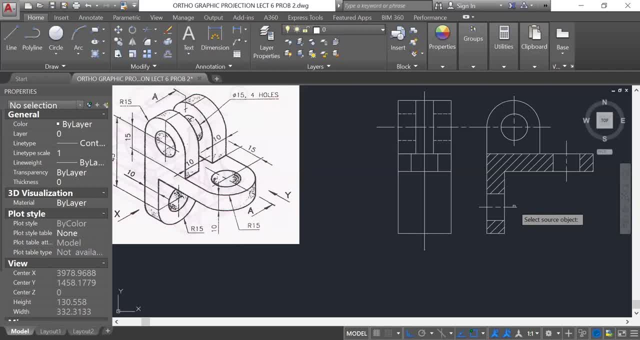 these vertical ones. these vertical ones are hidden lines, are hidden lines. end: Now we will consider the lowermost part, that is the centerline, that is anchor and adjust, Now construct. so this is a circle, so construct a circle and then another circle for the slot. 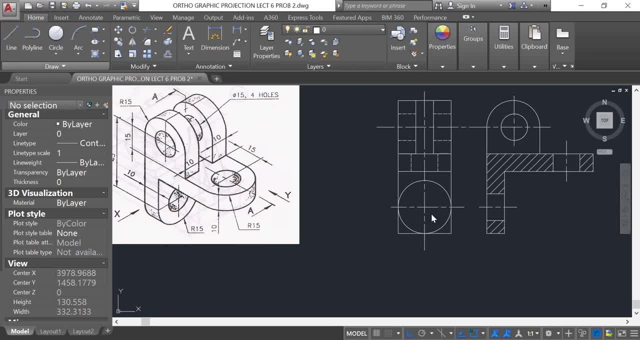 of radius 7.5 and then just go ahead and move this line, Just pick on the end point and just move it up. so every time you don't have to do that, Every time you don't have to do the trim. Now, for this circle, you do the trim. 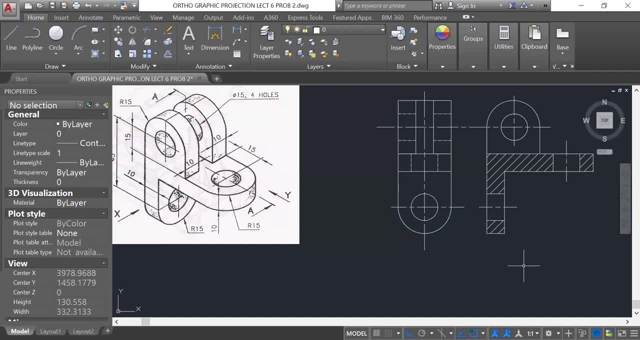 So that completes the right hand side. Right And Okay, Thank you, Bye, Bye, Bye. I can say: Now what is remaining is the top. Now, what remains is the top. So we have a top. I am going to do again, offset of 20.. 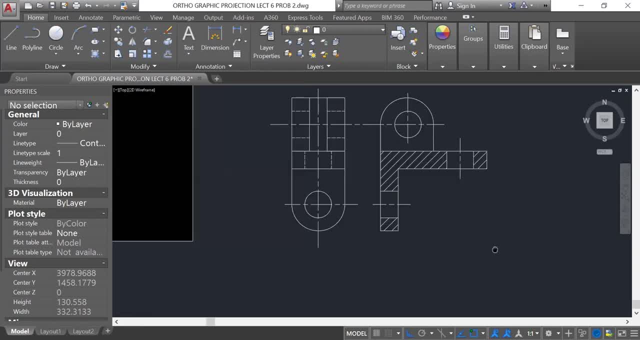 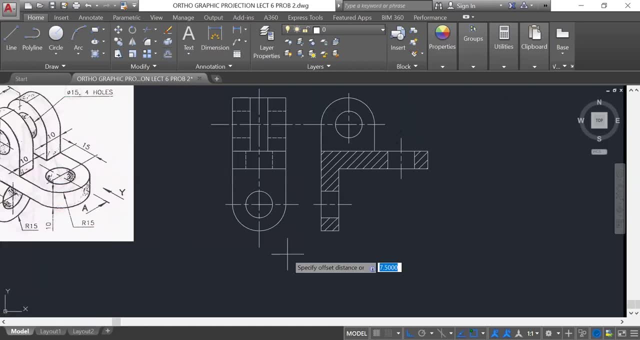 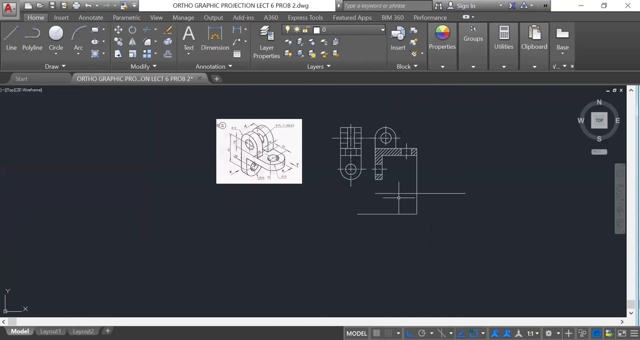 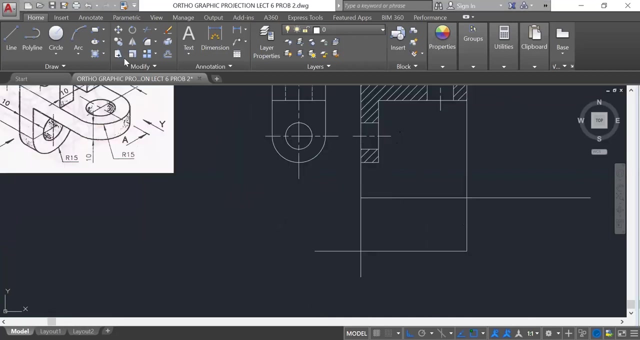 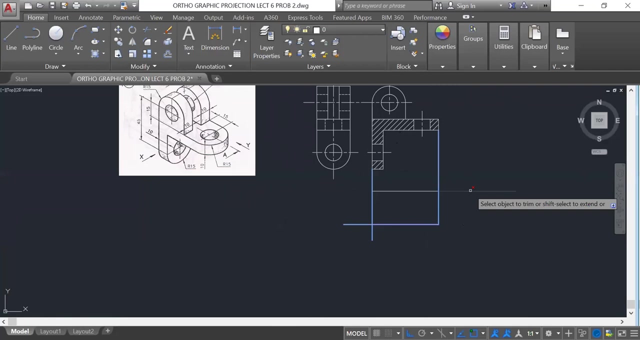 Okay, So we have a top now And Drop the projector. Width is 30. Trim out the excess lines. construct the center lines here rapidly. top view: one complete circle and one semicircle. semicircle will be complete. circle: the inner one. 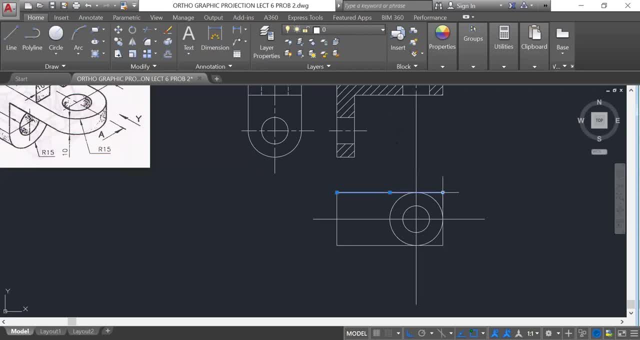 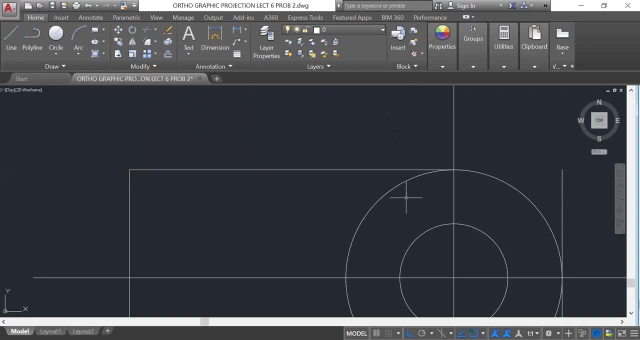 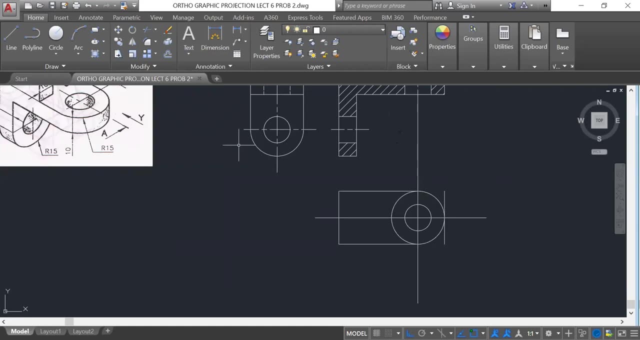 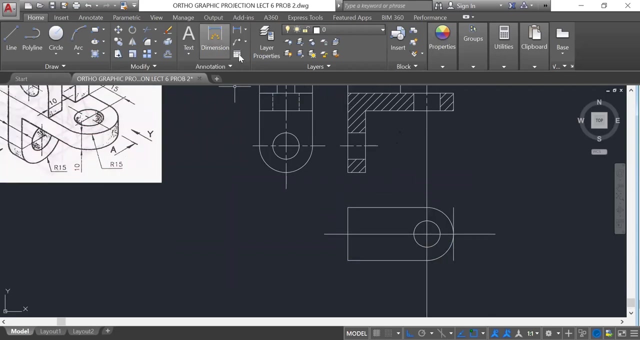 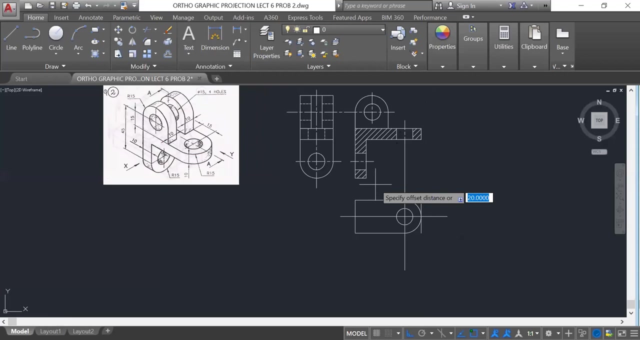 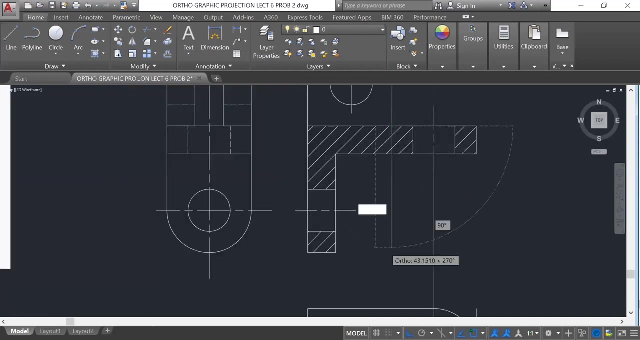 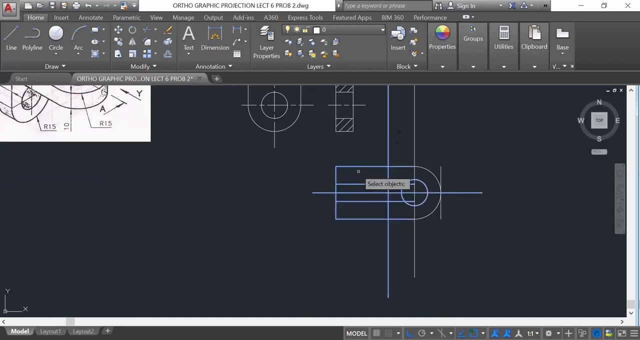 and the outer one. just do a trim on the circle like that, then do a offset for this two top plates. thickness of this plate is 10, 10, 1 and 2. right click enter and drop the projectors down. select this whole bunch right click. 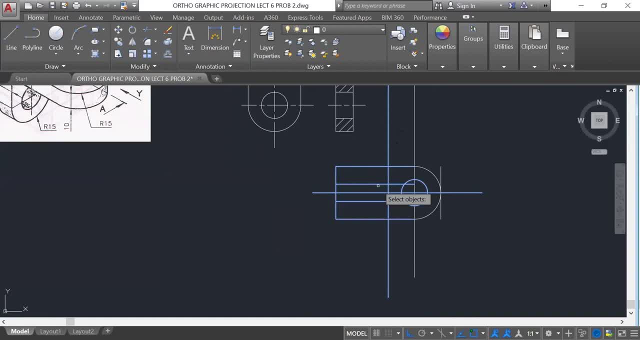 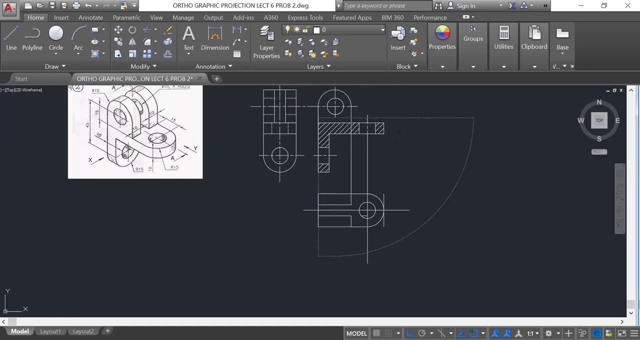 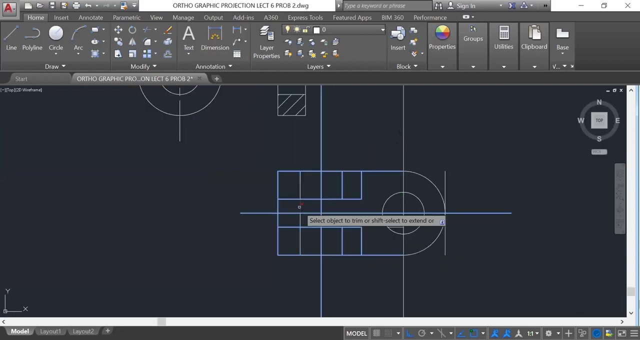 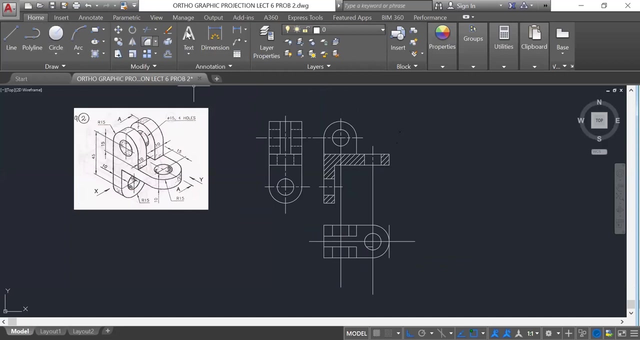 and frame one. select this, just that correct. correct and also center line. offset it 7.5 5, 5. that's it. right click enter and then just do a trim, enter and change this to hidden and change this to hidden match properties. tick 1. 2, 3, 4, 5, 6, 7, 8, 9, 10, 11, 12, 13, 14, 15, 16, 17, 18, 19, 20, 21, 22, 23, 24, 25, 26, 26. 27, 27, 28, 28, 29, 30, 31, 32, 33, 34, 35, 36, 37, 38, 39, 40, 41, 42, 43, 44, 45, 46, 47, 48, 49, 50. 51, 52, 53, 53, 53, 54, 55, 56, 57, 58, 59, 60, 61, 62, 63, 62, 63, 64, 65, 66, 67, 68, 69, 69, 70, 71. 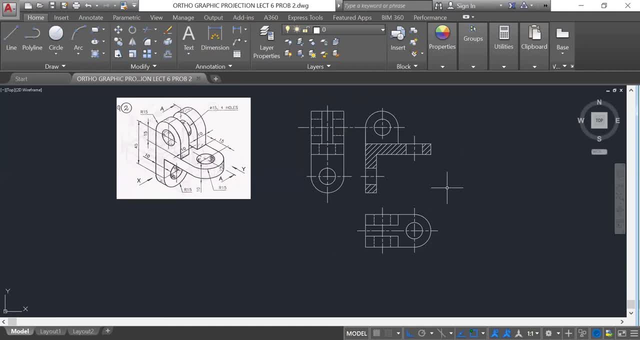 72, 73, 74, 75, 76, 76, 77, 78, 79, 80, 81, 82, 83, 84, 85, 86, 87, 88, 89, 90, 91, 92, 93, 93, 94, 95. 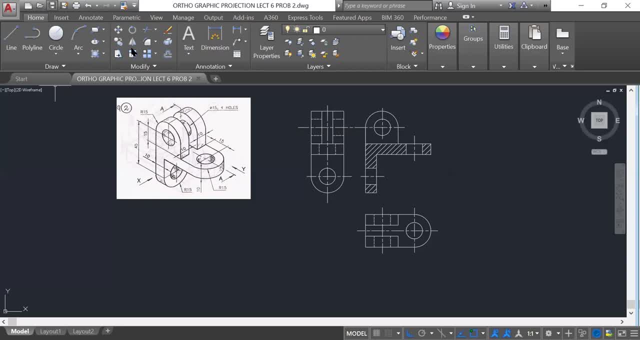 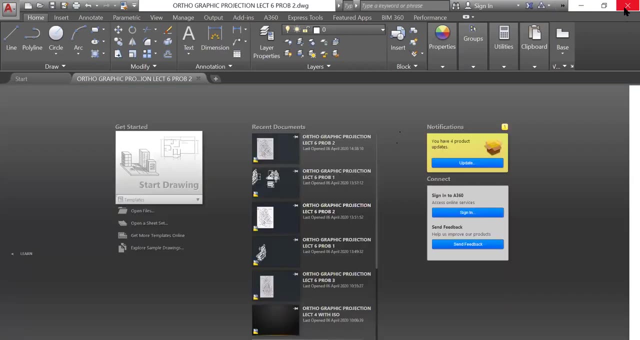 96, 97, 97, 98, 98, 99, 100, 100, 12, 13, 14, 15, 16, 17, 17, 18, 19, 20, 21, 22, 23, 24, 25, 26, 27, 28. 29, 30, 31, 32, 33, 33, 34, 35, 36, 37, 37, 38, 39, 41, 42, 43, 43, 44, 45, 46, 47, 48, 49, 50, 51, 52. 53, 53, 54, 55, 56, 57, 58, 59, 60, 61, 62, 63, 63, 64, 65, 66, 67, 68, 69, 69, 70, 71, 62, 63, 64, 65. 66, 67, 68, 68, 69, 69, 70, 71, 72, 73, 73, 74, 74, 75, 76, 76, 77, 78, 78, 79, 79, 80, 80, 80, 80, 80. 80, 81, 82, 83, 84, 85, 86, 87, 88, 89, 90, 91, 92, 93, 94, 95, 96, 97, 97, 98, 98, 99, 100, 10, 10, 11. 12, 13, 14, 15, 16, 17, 18, 19, 20, 21, 22, 23, 24, 25, 26, 27, 28, 29, 30, 31, 32, 33, 34, 35, 36, 37. 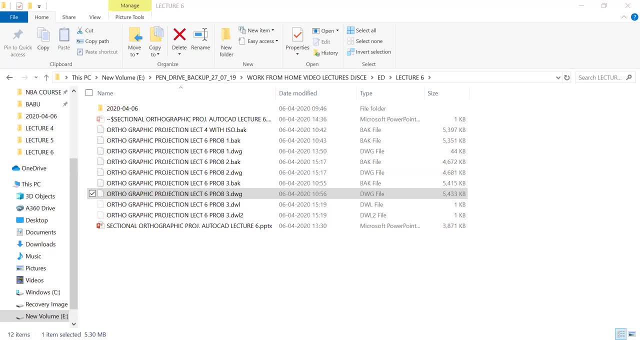 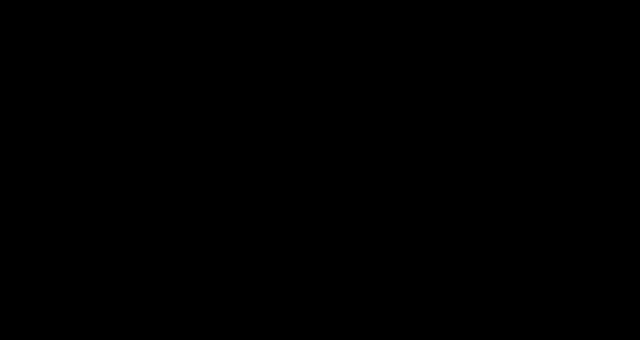 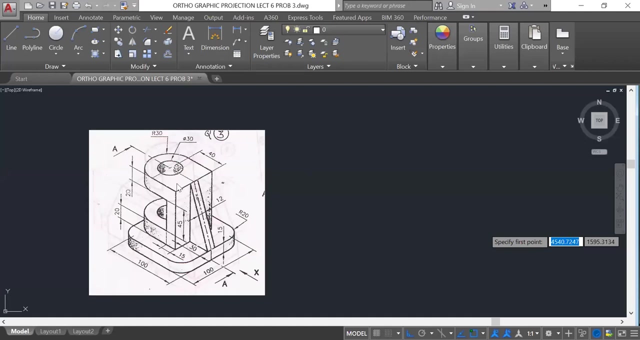 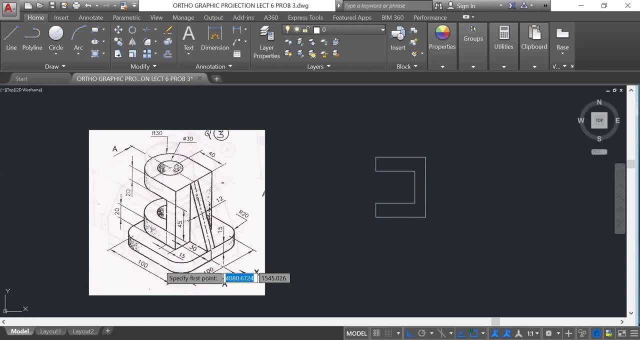 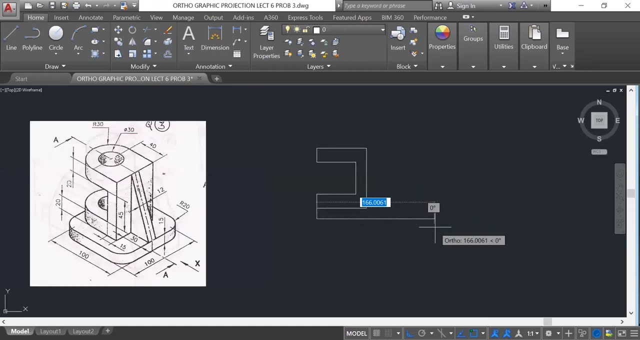 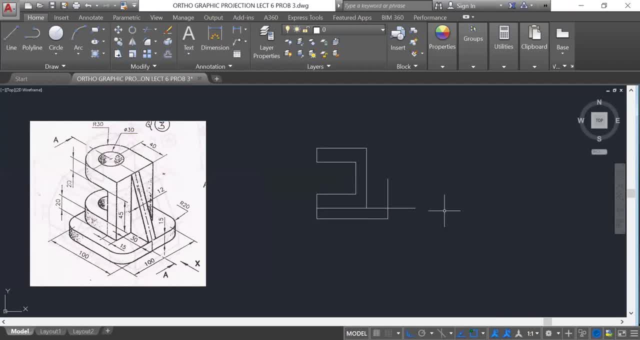 12, 13, 14, 15, 16, 17, 19, 20, 21, 23, Oh, and then go to trim like this. then there are the circular slots at a distance of 30 from the edge. all right, because the center is at 30. right, so do. 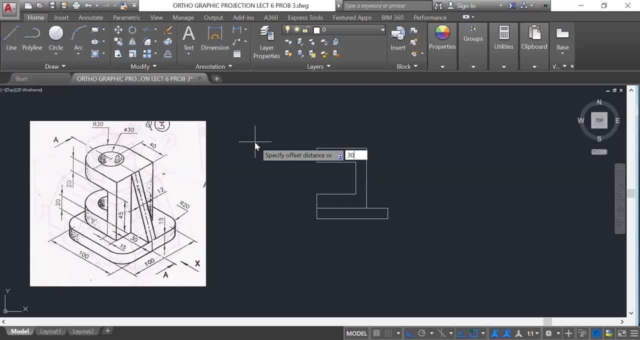 a quick offset by 30, one and enter- this will be your center line- and offset that by 50, because the diameter of the slot is 1, 2, right-click, enter this and then go on and trim all this stuff. right click: 1, 2, 3, 4, 5, 6, 7, 8, right click, enter and just delete. 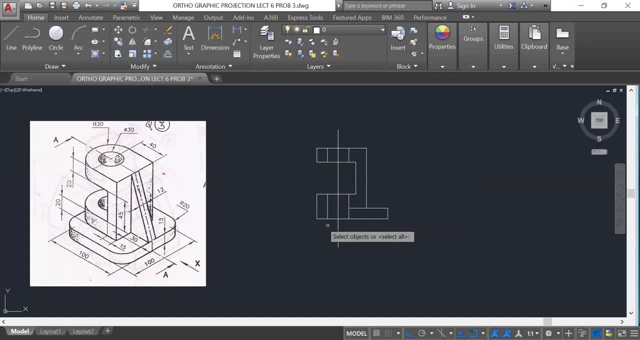 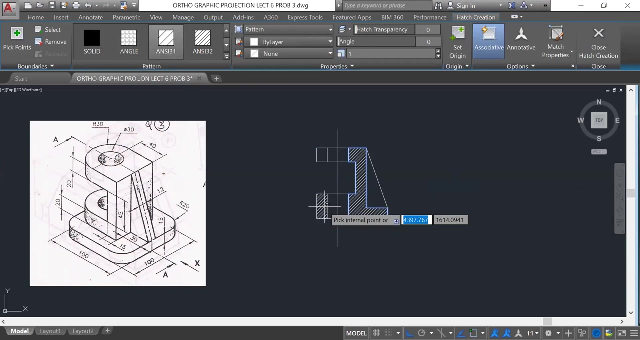 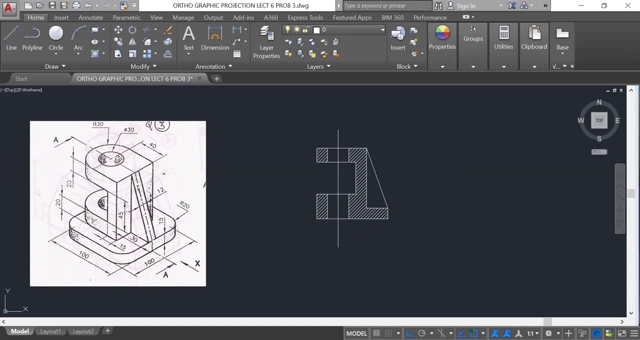 this and trim this edges. ok, alright, so now, only thing that is remaining is the rib. that will be this part. now, whatever is remaining is the hatching. so go to hatch and c 31 areas and right click, enter and that is your sectional side. alright, so I am just giving you some time. 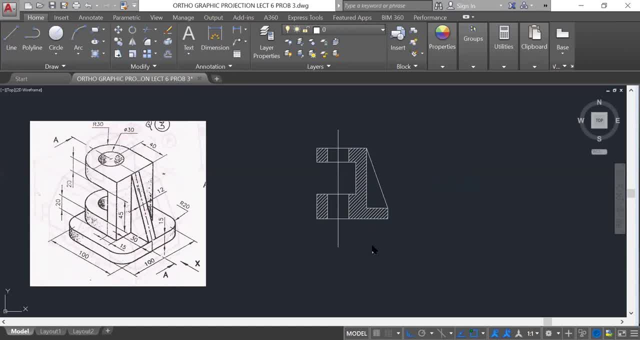 to think about it. So we have constructed the sectional side view without constructing a front view and top. All right, sectional side view through AA without constructing the front view and top view. This is done just by measurements of the diameter. Okay, let me just quickly take the attendance now. 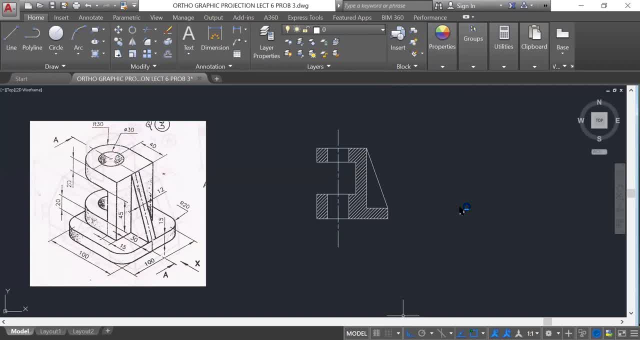 This is for the second lecture. Okay, There is a lot of room. Just see the space in the middle. Yes, anybody has any questions? Yes, sir, Yes, go ahead. Ask any students have any question. no, sir, okay, um. 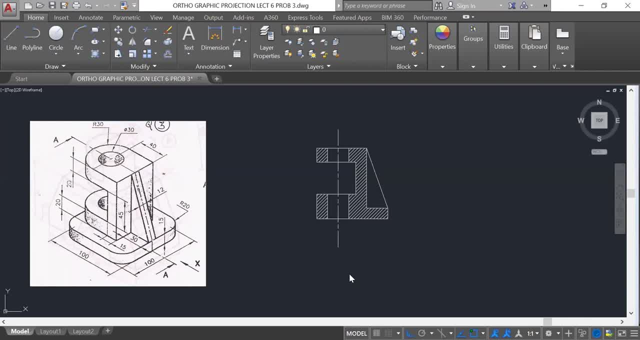 um, um, okay, all right, uh, a division of this e-division students have. is the solids projection of solids done for you? hello, hello, e-division students. is the projection of solids done for you? started a little bit, okay, so you know, if you want, uh, because i have. 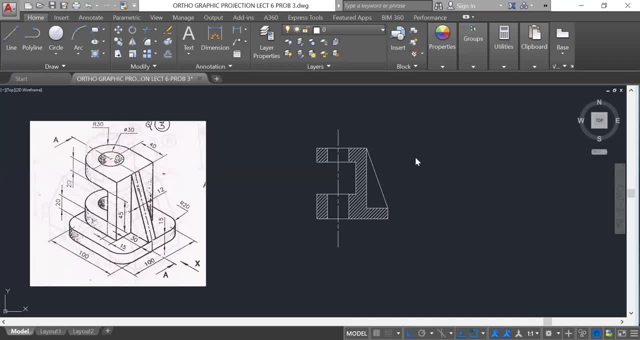 completed my six lectures. so you know, if i, if i feel anything is remaining, i will okay. so if i, if anything is remaining, i will just contact the students accordingly. you know i will schedule, so i will let you if any more lectures are available. all right, so i'm going to end the lecture. thank you.